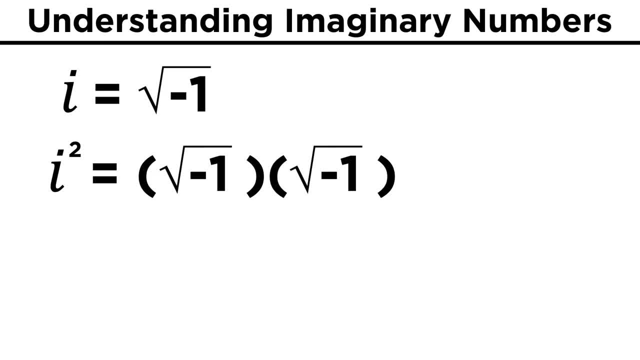 I squared, for example, is root negative one times root negative. one which is negative one, I cubed- can be expressed as I squared, I squared times I, and we just said I squared is negative one, so I cubed is equal to negative. 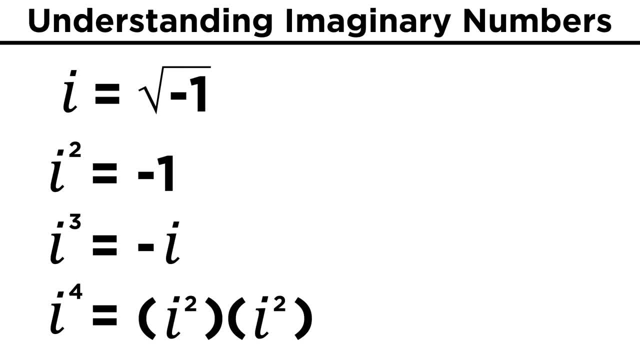 I. I to the fourth: is I squared times I squared, or negative one times negative one, which is one? This series of four values repeats every four powers of I. so I, to the fifth through eighth, will be these values once more. and then we start again. 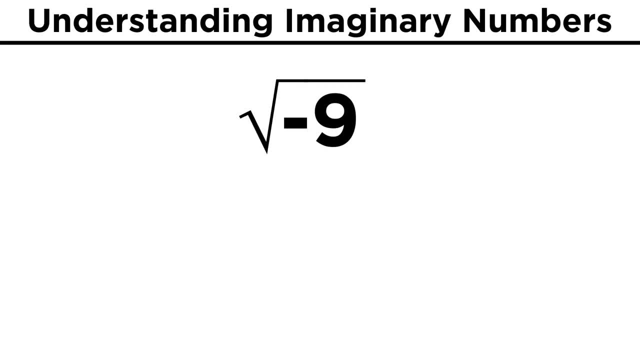 I can also be fixed. Here's the problem we found with other numbers. Take the square root of negative nine, for example. This can be expressed as root nine times negative one, and therefore root nine times root negative one. Root nine is three and root negative one is I, so we get three. I. 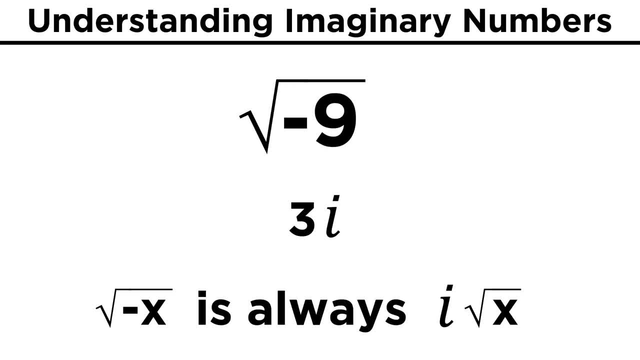 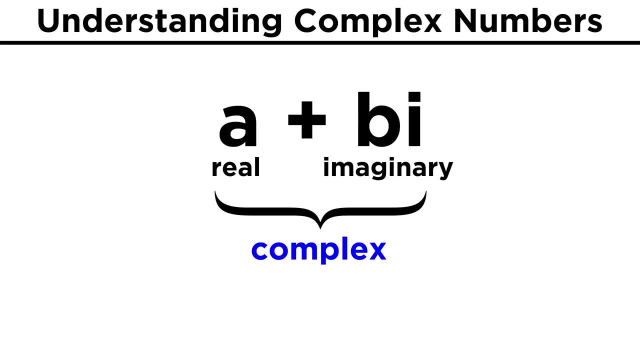 In this way, the root of negative X will always be I root X. Any time we have imaginary numbers together with real numbers, they are always equal. I root X equals two numbers. they are called complex numbers and we write them in the form of A plus BI. 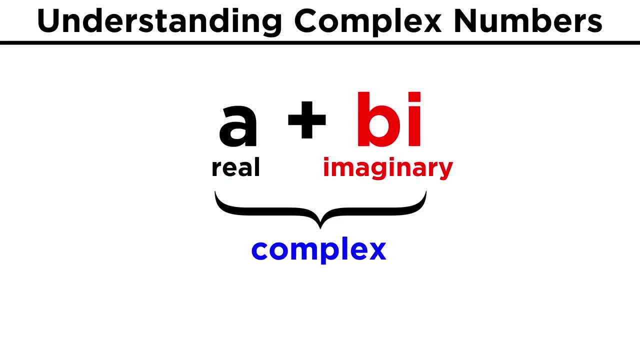 Complex numbers have a real part, that's the A, and then an imaginary part, which is BI. In this way, all numbers are technically complex numbers because if B is zero, the imaginary part goes away and we just have a real number. 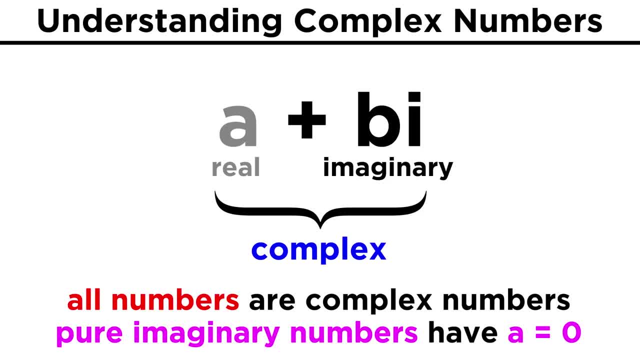 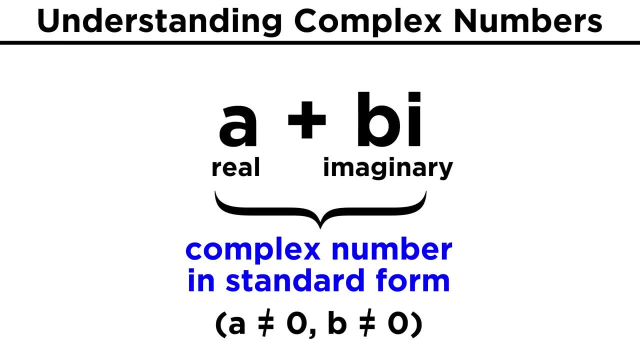 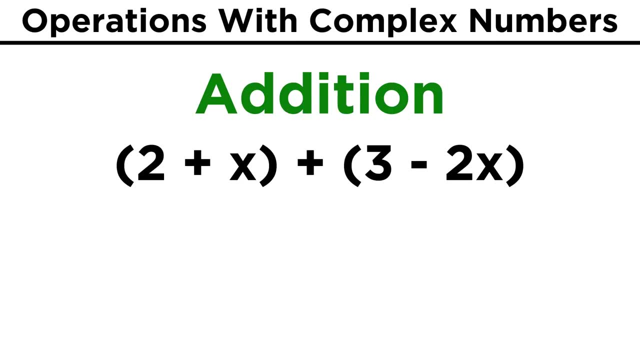 If A is zero, we have a pure imaginary number, as there is nothing real about it. But if A and B are both nonzero, we have a complex number in its standard form. We can do operations with complex numbers just like we would if I was some variable. 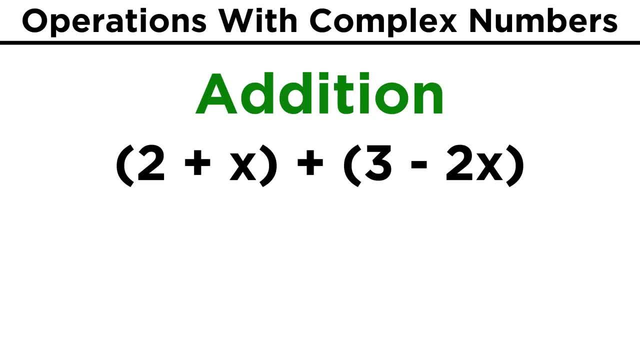 like X. If we had the quantity two plus X plus the quantity three minus two X, we would add the numbers together to get five And add the X's together to get negative X. It's exactly the same with I. so if we change these X's to I's, we get five minus. 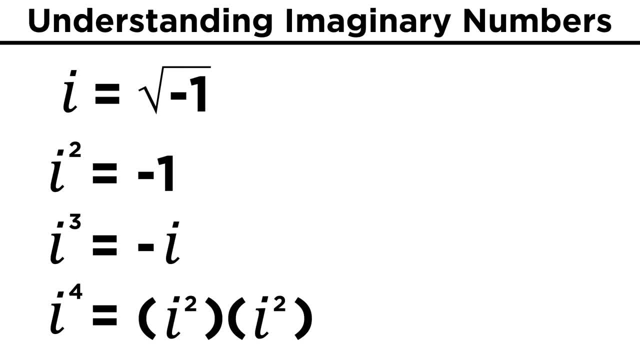 I. I to the fourth: is I squared times I squared, or negative one times negative one, which is one? This series of four values repeats every four powers of I. so I, to the fifth through eighth, will be these values once more. and then we start again. 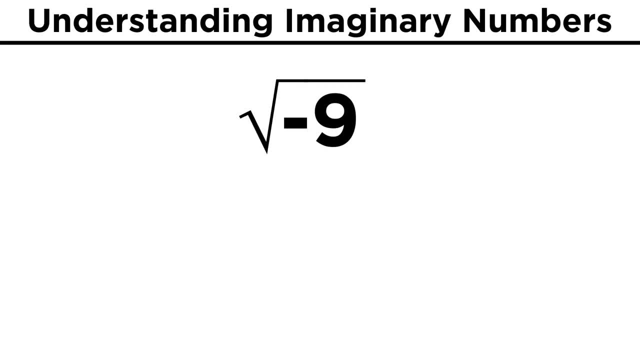 I can also be fixed. I can also be found with other numbers. Take the square root of negative nine, for example. This can be expressed as root nine times negative one, and therefore root nine times root negative one. Root nine is three and root negative one is I, so we get three I. 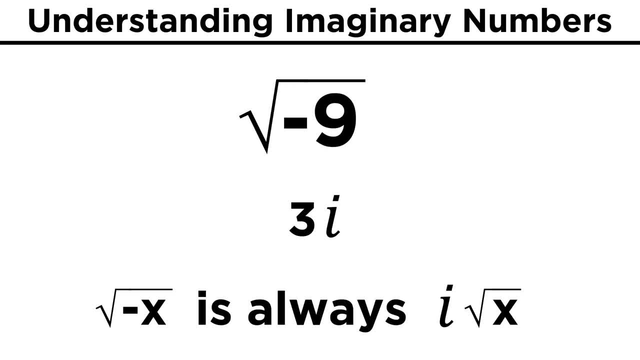 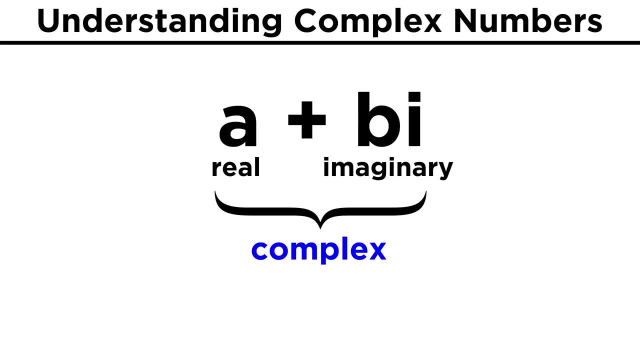 In this way, the root of negative X will always be: I root X. Anytime we have imaginary numbers together with real numbers, they are always an imaginary numbers. they are called complex numbers and we write them in the form of A plus BI. 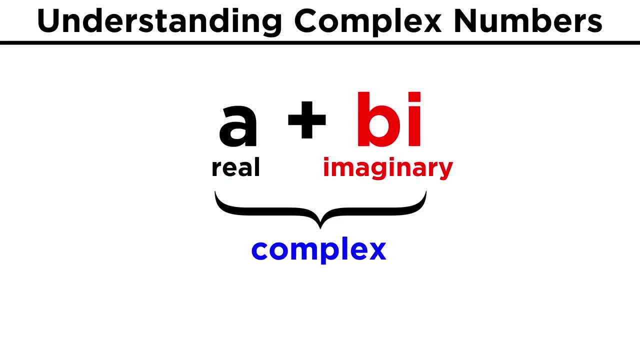 Complex numbers have a real part, that's the A, and then an imaginary part, which is BI. In this way, all numbers are technically complex numbers because if B is zero, the imaginary part goes away and we just have a real number. 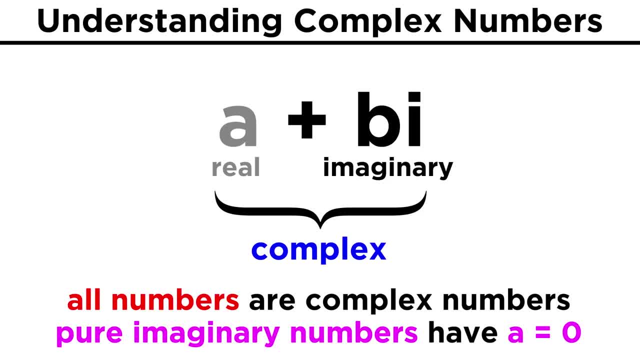 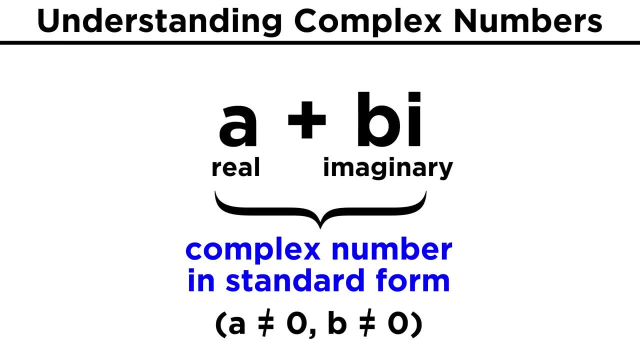 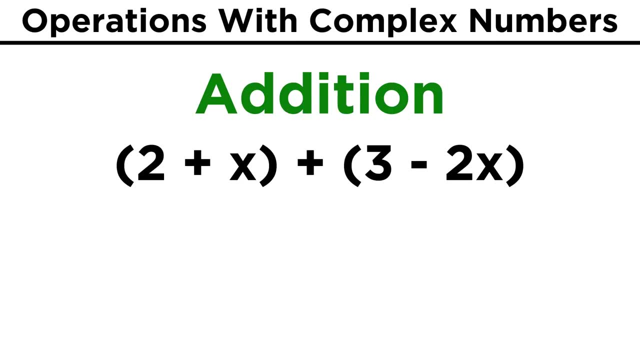 If A is zero, we have a pure imaginary number, as there is nothing real about it. But if A and B are both nonzero, we have a complex number in its standard form. We can do operations with complex numbers just like we would if I was some variable. 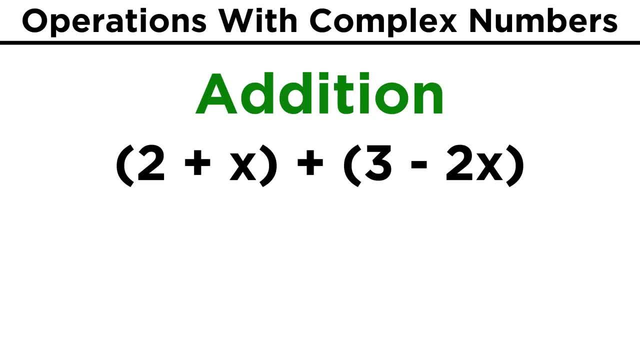 like X. If we had the quantity two plus X plus the quantity three minus two X, we would add the numbers together to get five And add the X's together to get negative X. It's exactly the same with I. so if we change these X's to I's, we get five minus. 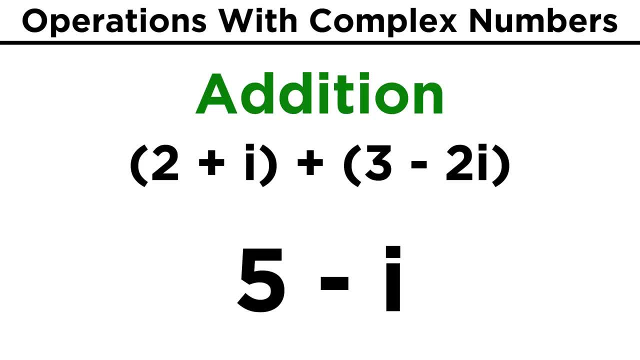 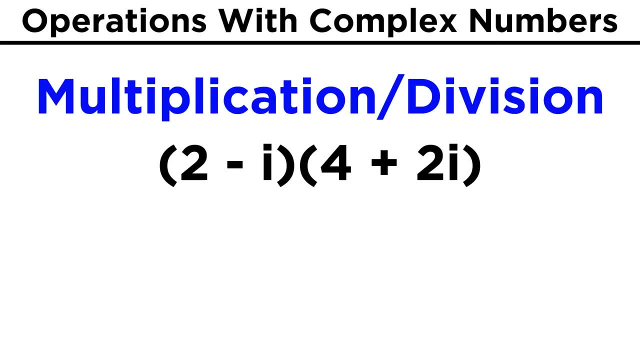 I. Since we already know how to do this, we won't need to practice. Multiplication and division work the same way, with just one extra twist. We have to remember that I squared equals negative one, so let's say we have the quantity. 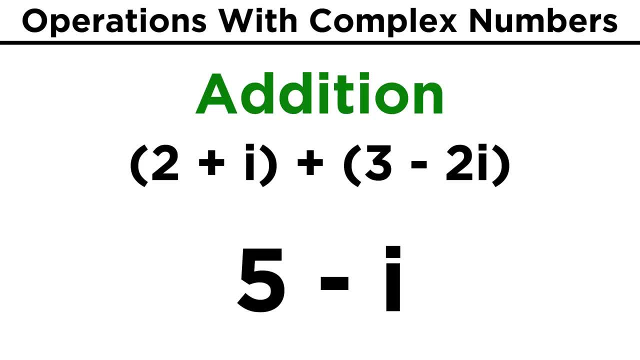 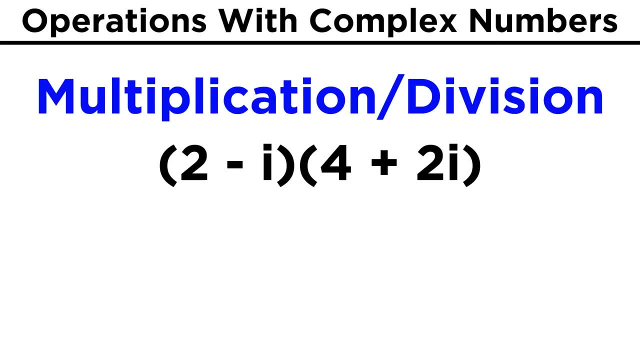 I. Since we already know how to do this, we won't need to practice. Multiplication and division work the same way, with just one extra twist. We have to remember that I squared equals negative one, so let's say we have the quantity. 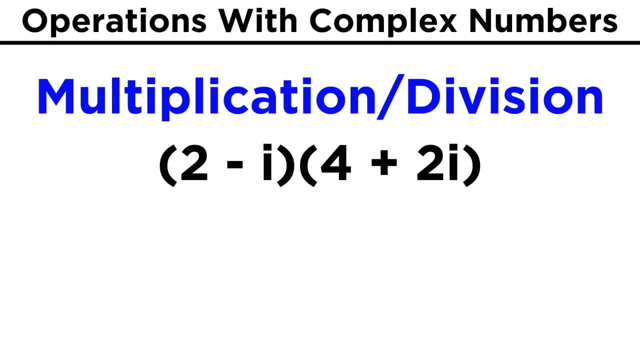 two minus I, times the quantity four plus two. Okay, We can just FOIL this exactly the way we would with two binomials: First gives eight, Outer gives four I. inner gives negative four, I. and last gives negative two, I squared. 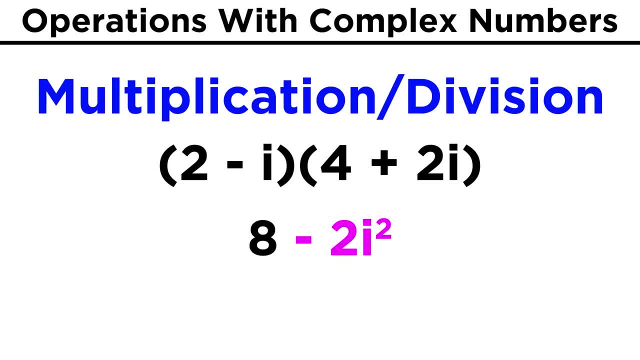 The two I terms cancel each other out. and negative two, I squared, is negative two times negative one, which is two. so we get eight plus two or ten. This is how complex numbers cancel out. Now let's look at other problems. 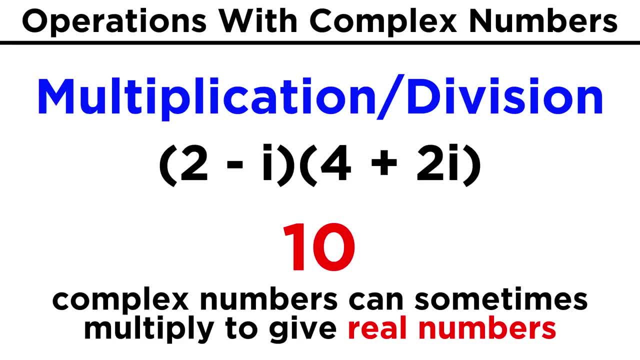 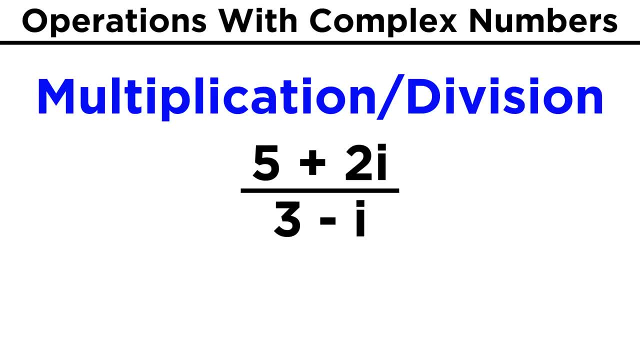 Complex can sometimes multiply to give real numbers. This fact will come in handy if we want to divide complex numbers. Take something like five plus two i over three minus i. Obviously we can't do much with this as it is, but if we had a real number in the 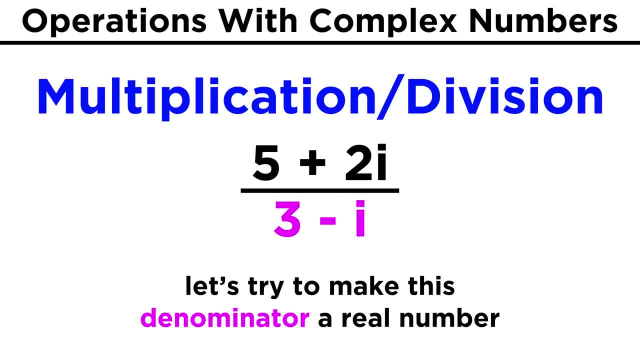 denominator. we could do something, As we just learned: it is possible to multiply complex numbers to get a real number. so we can multiply the top and bottom of this quotient by the same complex number to do exactly that. But what will this complex number be? 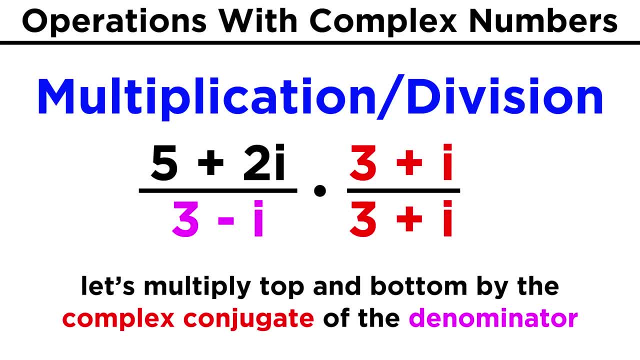 As it turns out, we will always get a real number when we multiply a complex number by its complex conjugate. The complex conjugate of a complex number is just the same number, but with the sign in between the two terms reversed. So in this case we want to multiply the top and bottom of this quotient by the same complex. 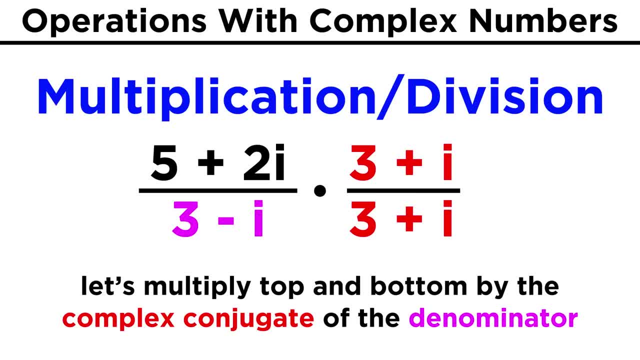 number. So we can multiply the top and bottom by three plus i. If this had been a plus, we would use a minus instead, But now we can FOIL the bottom and the top. Let's do the top first. Fifteen plus five, i plus six, i plus two, i squared. 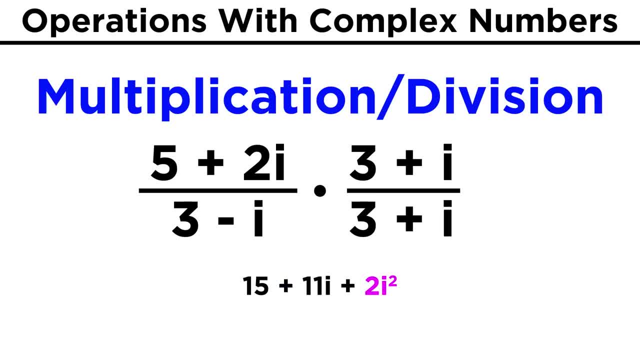 We combine these to get eleven: i two i squared becomes negative two and we end up with thirteen plus eleven i. Then on the bottom we get nine plus three. So we have nine plus three. i minus three. i minus i squared. 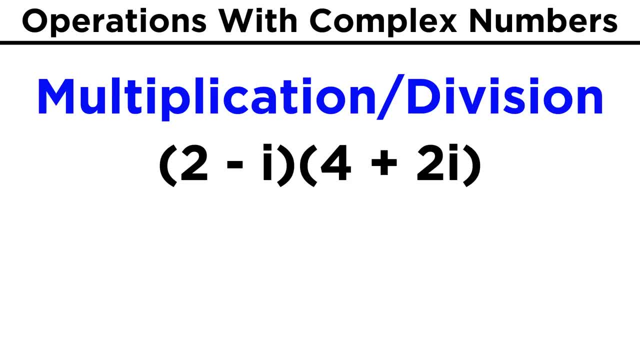 two minus I, times the quantity four plus two. Okay, So we'll just save this one for next time. We can just foil this exactly the way we would with two binomials: First gives eight, Outer gives four: I. inner gives negative four, I. and last gives negative two, I squared. 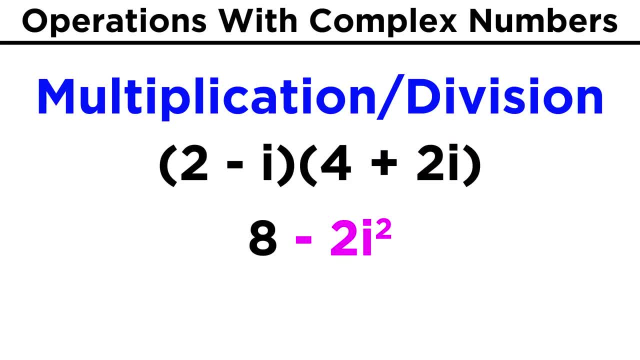 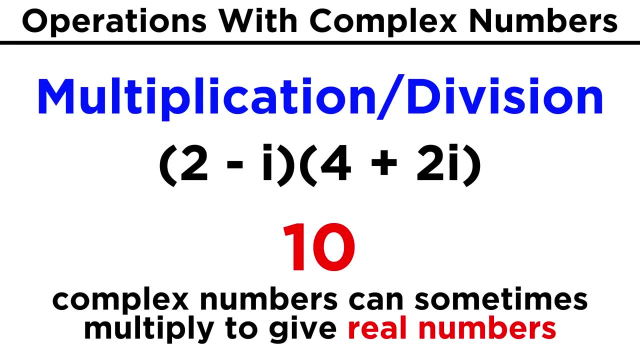 The two I terms cancel each other out and negative two. I squared is negative two times negative one and that's two. so we get eight plus two or ten. This is how complex numbers can work. Thank, you can sometimes multiply to give real numbers. 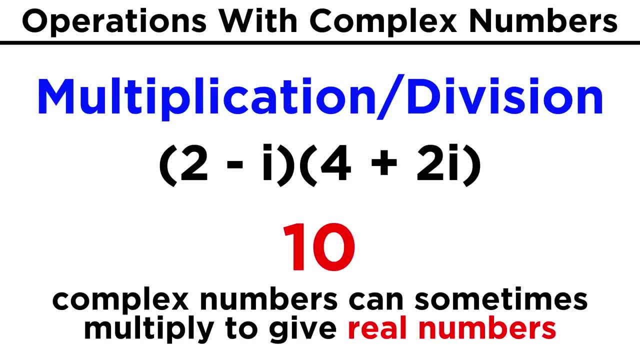 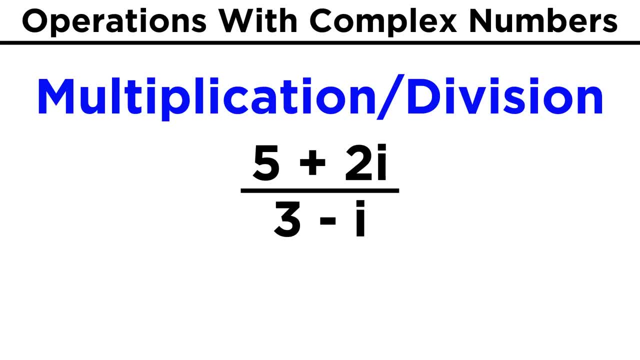 This fact will come in handy if we want to divide complex numbers. Take something like five plus two i over three minus i. Obviously we can't do much with this as it is, but if we had a real number in the denominator we could do something. 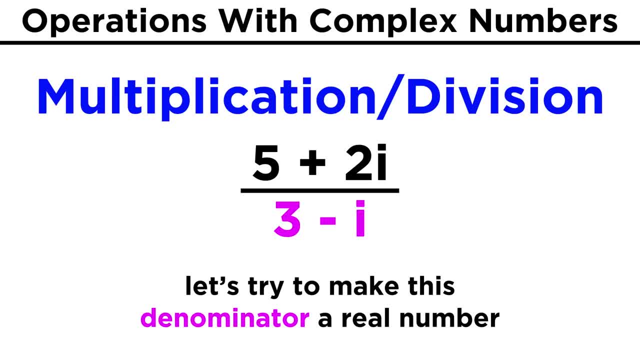 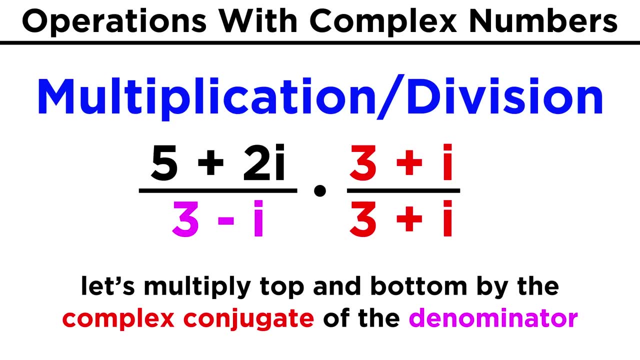 As we just learned, it is possible to multiply complex numbers to get a real number. so we can multiply the top and bottom of this quotient by the same complex number to do exactly that. But what will this complex number be? As it turns out, we will always get a real number when we multiply a complex number by. 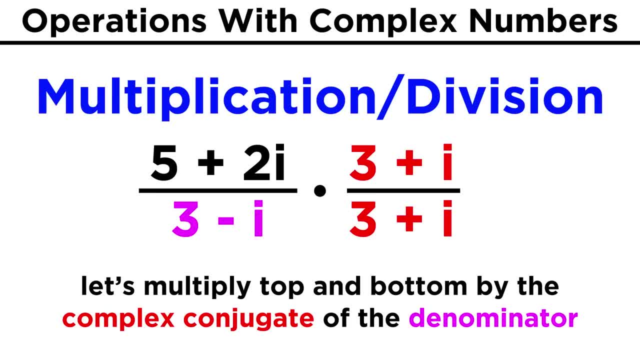 its complex conjugate. The complex conjugate of a complex number is just the same number, but with the sign in between the two terms reversed. So in this case we want to multiply the top and bottom of this quotient by the same complex number. 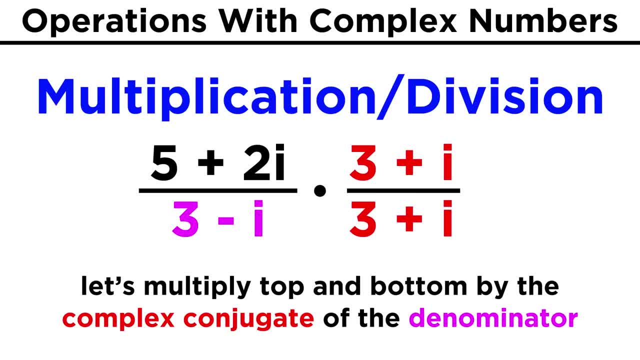 So we can multiply the top and bottom by three plus i. If this had been a plus, we would use a minus instead, But now we can FOIL the bottom and the top. Let's do the top first. Fifteen plus five, i plus six, i plus two, i squared. 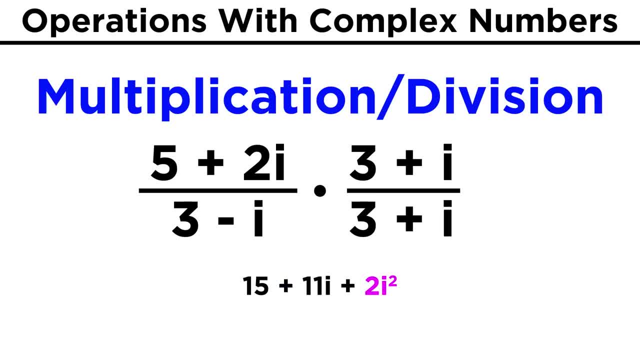 We combine these to get eleven: i two i squared becomes negative two and we end up with thirteen plus eleven i. Then on the bottom we get nine plus three plus i. Then on the top we get nine plus three. i minus three, i minus i squared. 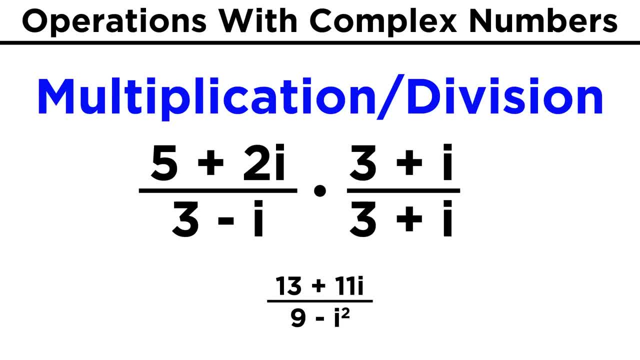 We notice that the i terms cancel out, which was exactly the plan, and this will always be the case. when we multiply complex conjugates, The negative i squared becomes positive one, leaving us with ten. Then we can just express this in standard form by splitting it up into two fractions. 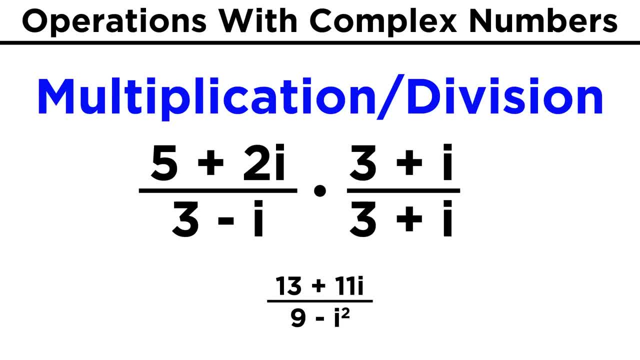 We notice that the i terms cancel out, which was exactly the plan, and this will always be the case. when we multiply complex conjugates, The negative i squared becomes positive one, leaving us with ten. Then we can just express this in standard form by splitting it up into two fractions. 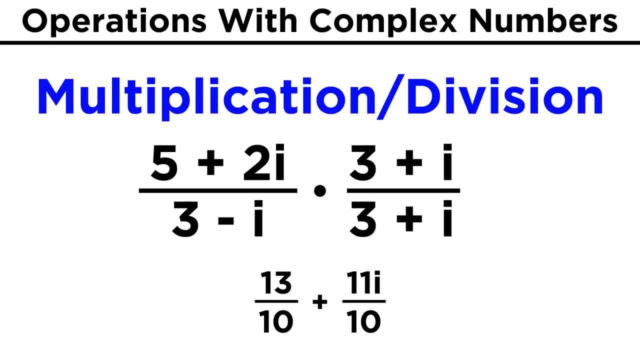 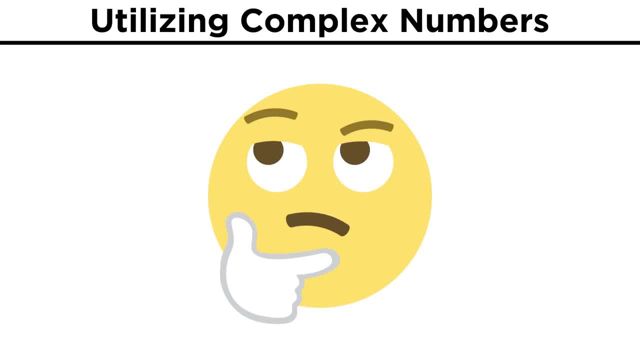 thirteen over ten plus eleven, i over ten, And even though it's a little messy, that's the way we divide complex numbers. Where might we see complex numbers? Well, remember, when we were finding solutions to polynomials, we would sometimes use the. 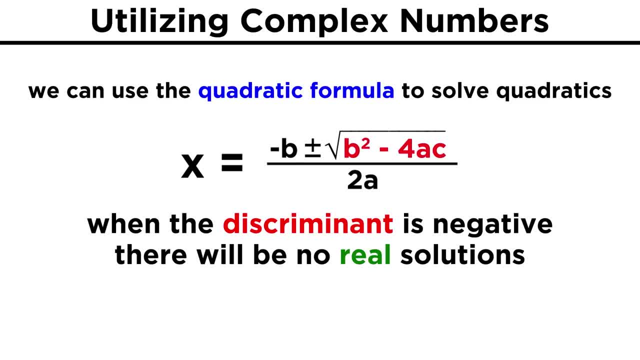 quadratic formula. But if the number under the radical or the discriminant turned out to be negative, we said that there were no solutions. Well, in truth, there were no real solutions. We can get imaginary roots If we express them in terms of: i. 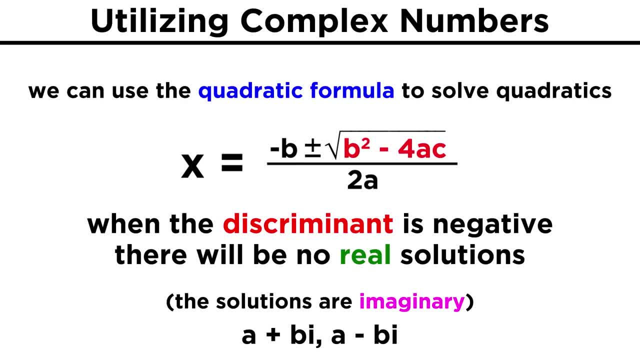 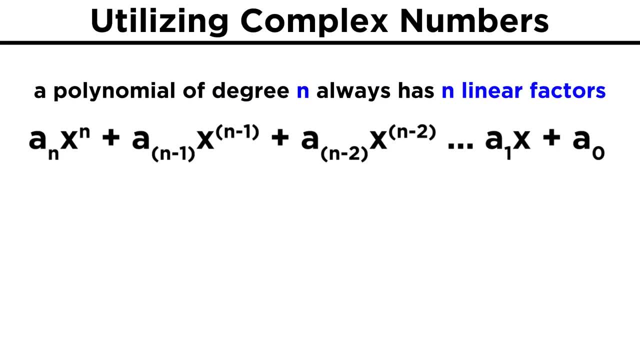 For quadratics with no real solutions, there will be two solutions in the form of complex numbers, and they will specifically be complex conjugates. In this way, a polynomial of degree n will always have n linear factors. There can be repeats, so they aren't always all unique. 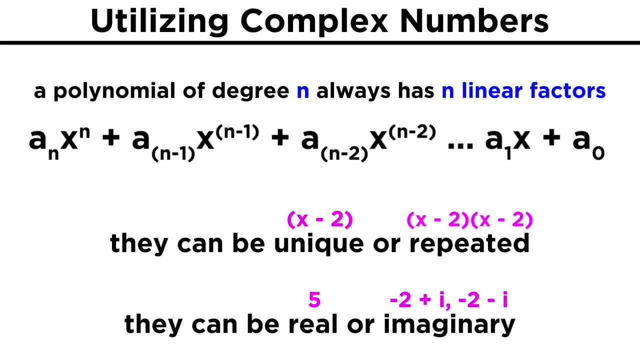 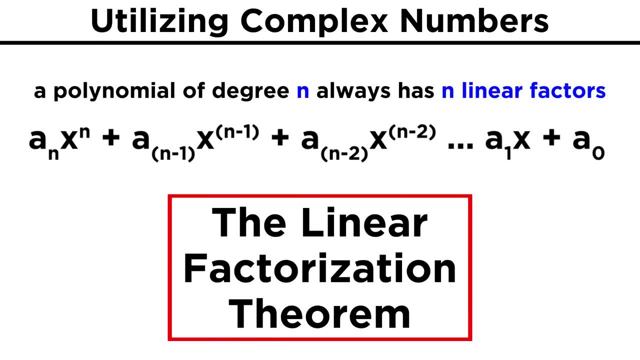 They aren't always all real numbers either. Some could be pairs of complex conjugates, as we just saw with the quadratic. If we take all of these into account, an nth degree polynomial will always have n linear factors. This truth is known as the linear factorization theorem. 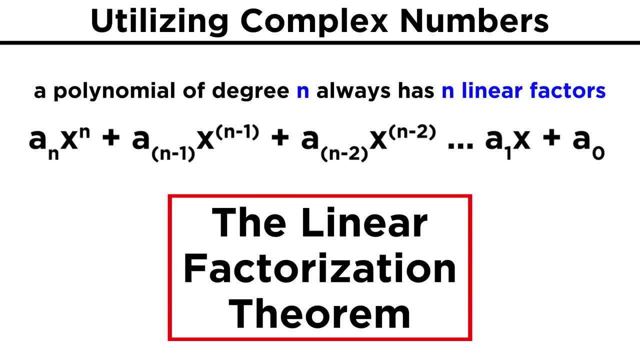 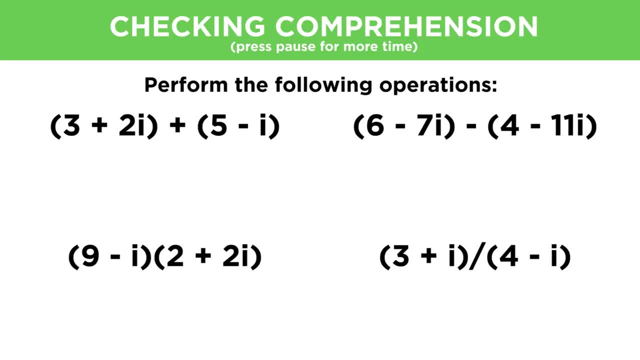 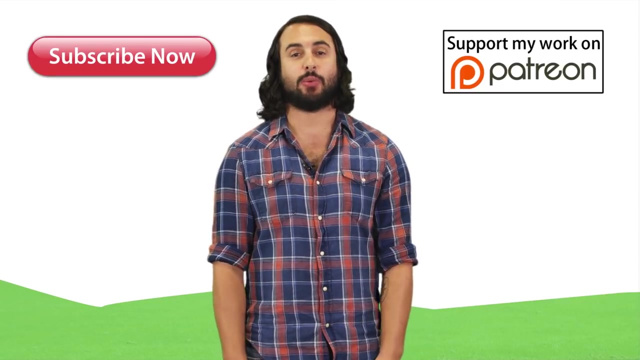 Complex numbers are very important in math, so let's check comprehension. Thanks for watching, guys. Subscribe to my channel for more tutorials. Support me on Patreon so I can keep making content And, as always, feel free to email me professordaveexplains at gmail dot com. I'll see you next time. Bye-bye.